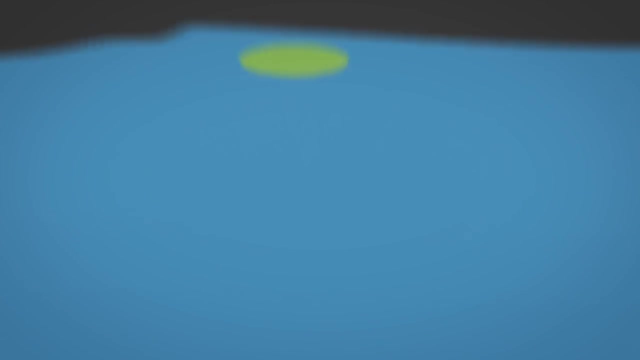 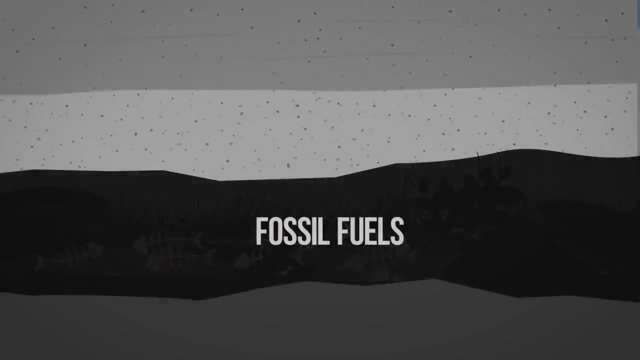 with swamps filled with organisms and plants. As they died, they sank to the bottom of swamps and oceans and, over millions of years, started decomposing under layers of sand, clay and other minerals. Different types of fossil fuels formed, depending on the combination of organic 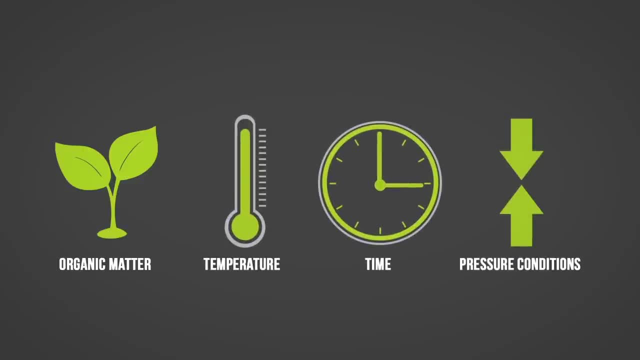 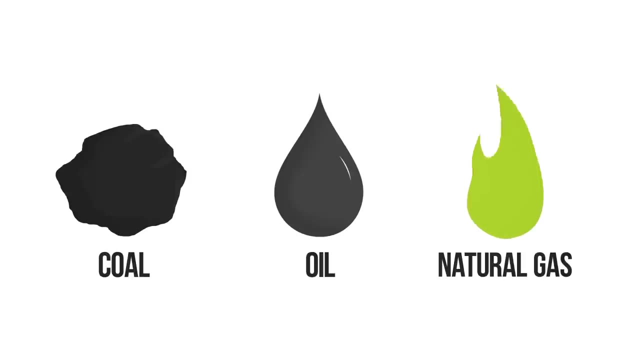 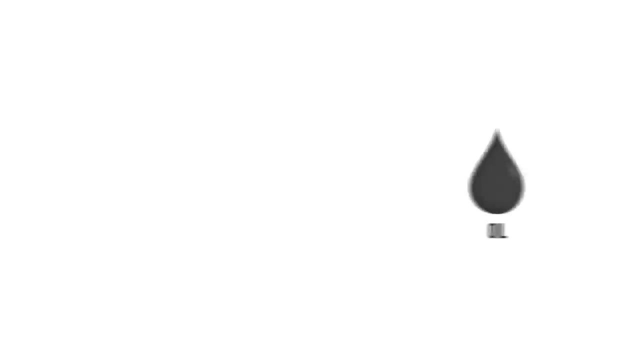 matter temperature, time and pressure conditions while decomposing. There are three major types of fossil fuels: coal, oil and natural gas. Coal was formed from ferns, plants and trees which hardened due to pressure and heat. Oil was formed from small organisms like zooplankton and algae. 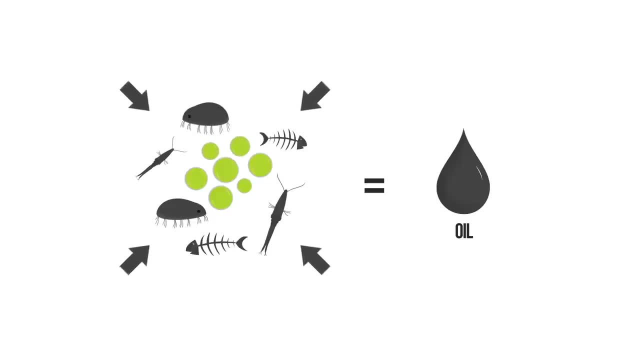 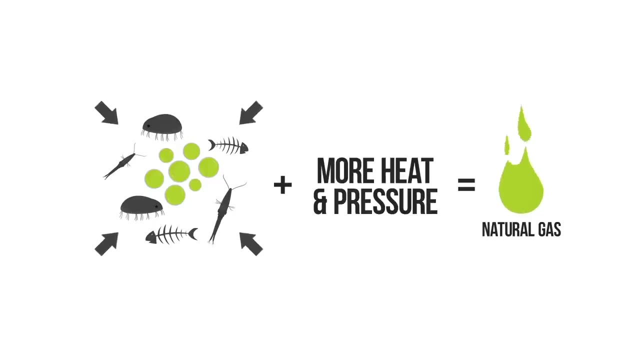 where pressure caused the more complex organic matter to decompose. Natural gas was formed by the same process as oil, only it was exposed to more heat and pressure, causing it to further decompose and turn into a gaseous form. Fossil fuels are sought after. 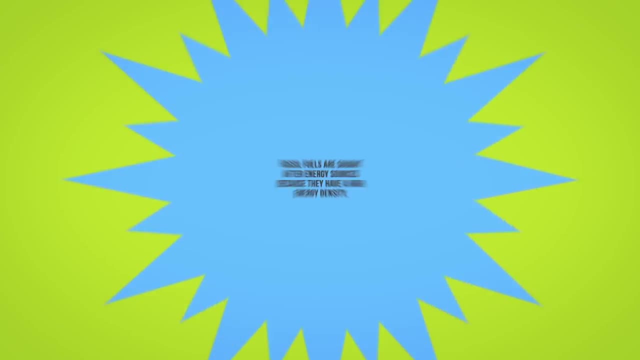 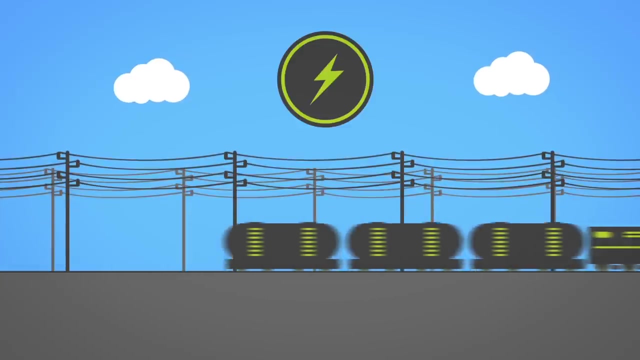 energy sources. because they have a high energy density, They are the world's dominant energy source. Fossil fuels have a variety of applications, from electricity production to transport fuels. They can also be used to make a variety of common products, from plastics to cosmetics, to even some. 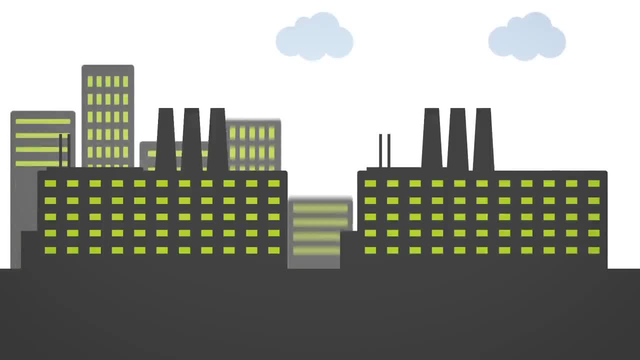 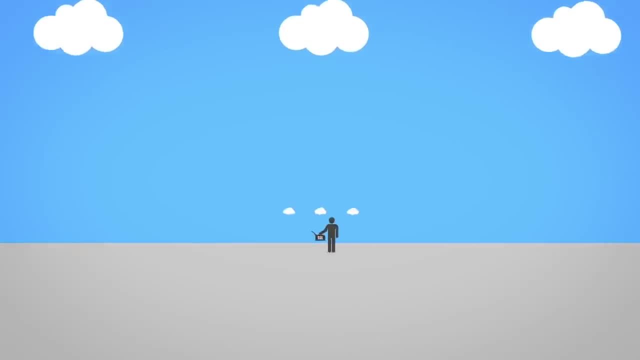 medicines. These were used to make the most efficient and efficient energy sources. The resources have powered industrialization over history and continue to do so today. Fossil fuels can be an abundant and cheap, or, in some cases, a scarce and expensive form of energy. 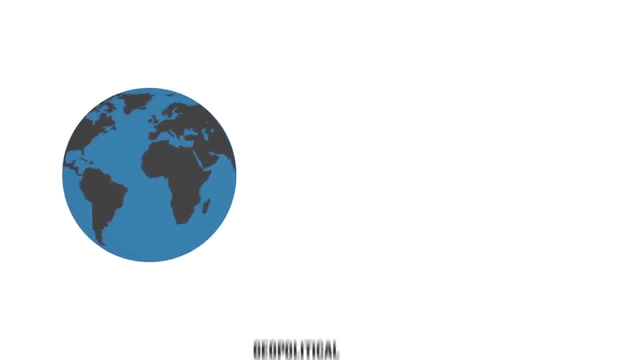 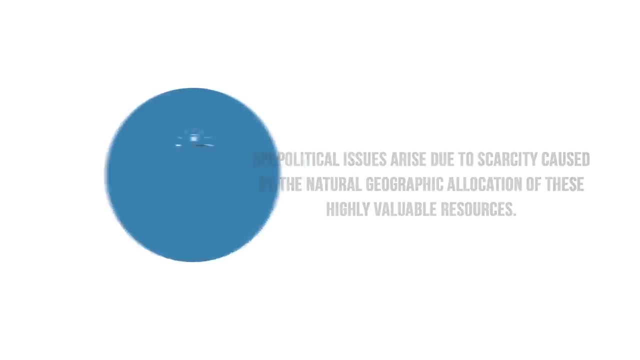 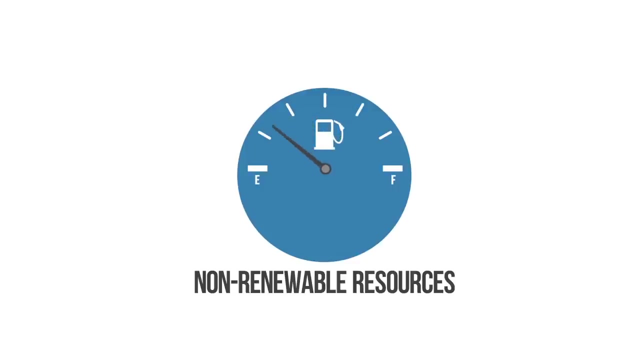 depending on geographic location. For this reason, geopolitical issues arise due to scarcity caused by the natural geographic allocation of these highly valuable resources. Fossil fuels are considered non-renewable resources because they take millions of years to form, which means that once they are used, the resources will not be replenished in a human lifetime. 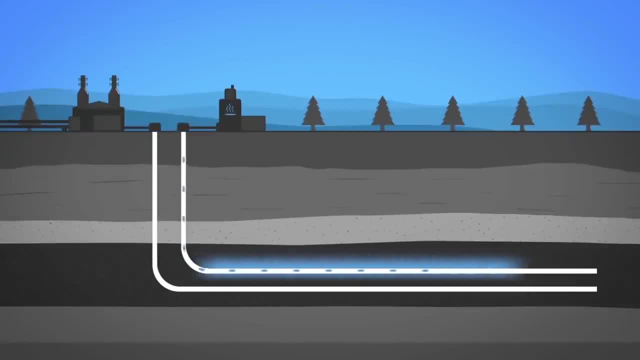 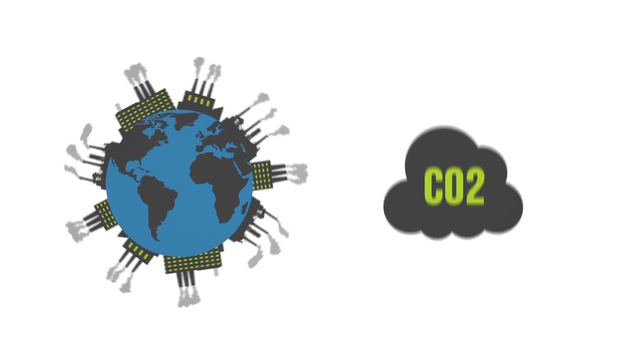 but will be reused. The gradual depletion of the most accessible fossil fuel reserves have forced companies to develop technologies for extracting more challenging or unconventional reserves. In many cases, this means additional safety and environmental concerns, as well as higher costs. Fossil fuels are also the largest emitters of carbon dioxide, a greenhouse gas which causes 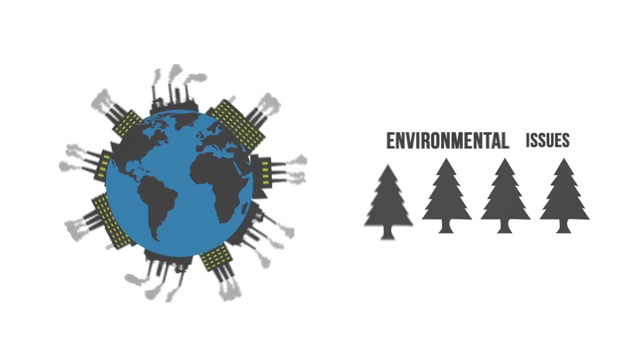 climate change. In addition, their production causes both environmental and human health issues. These concerns have triggered society to look at alternate sources of energy. Fossil fuels are also the largest emitters of carbon dioxide, a greenhouse gas, which causes climate change. These concerns have triggered society to look at alternate sources of energy that are more 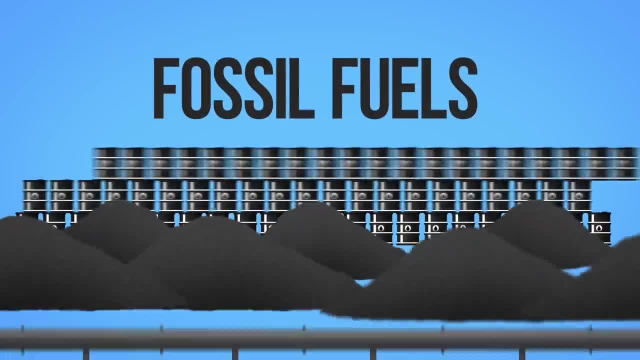 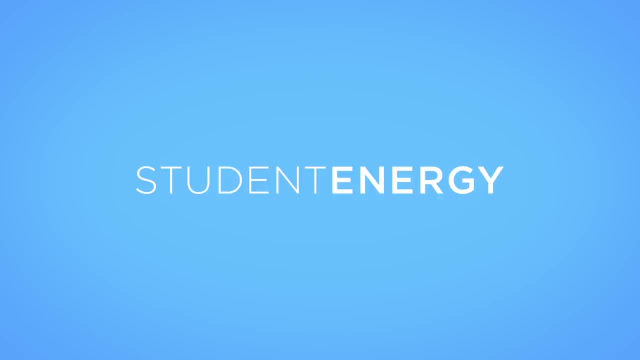 environmentally sustainable and renewable, That's fossil fuels.